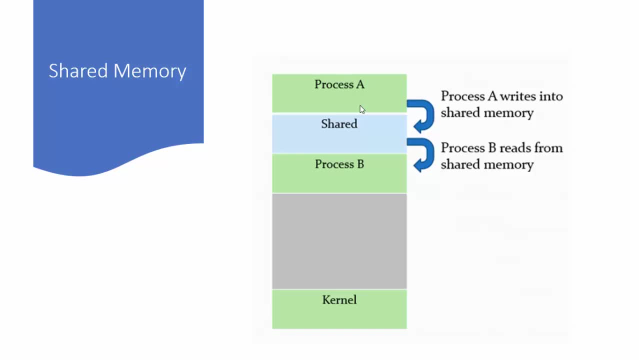 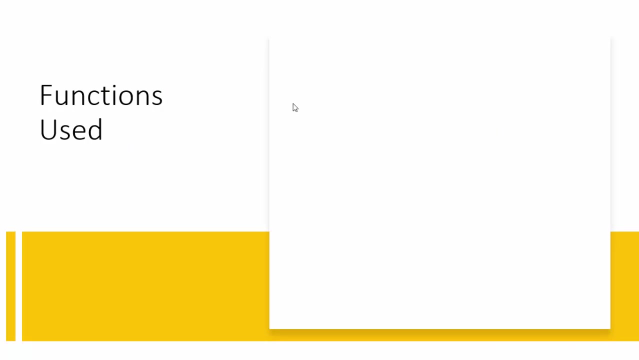 then the sender can write some data into the shared segment. Similarly, the receiver will first attach itself to the shared segment and then read data from the shared segment. For writing the programs for the shared segment, we need to use two very important functions. 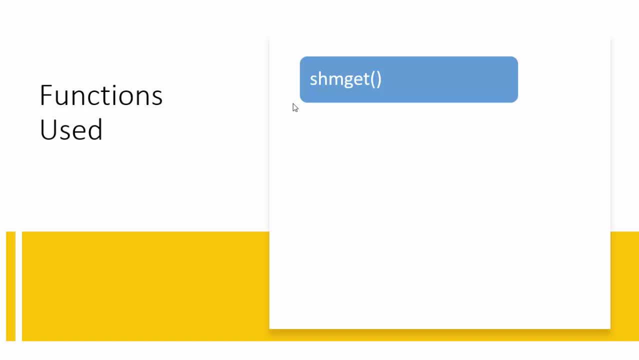 First one is shmget, So shared memory get. This function is used to create the shared memory segment. The second function is shmat- Shared memory attach. This function is used to attach the shared segment with the address space of the process. Until and unless we attach the shared segment with the address space of the process, 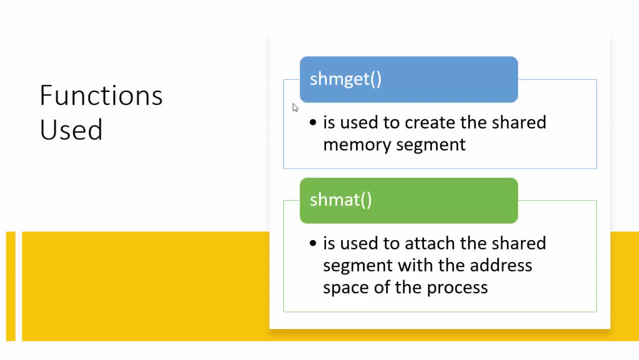 we cannot use that shared segment. Okay, it is just like until and unless you attach the pen drive to your system, you cannot use the pen drive. Okay, so we have to attach the shared segment to the address space. Another way to understand this is: a process cannot read or write data beyond the address space that is allocated to it. 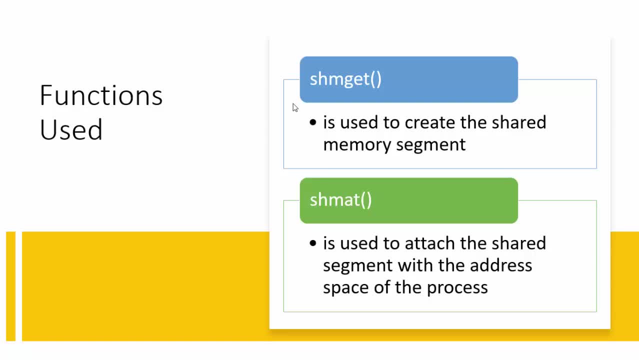 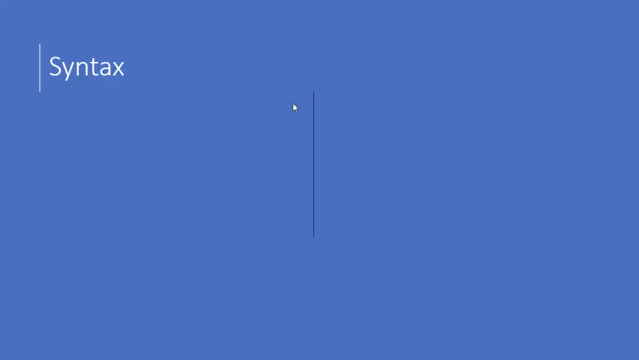 If I want to write or read into the shared segment, which is an external memory area that does not belong to the address space of the process. So we have to attach that shared segment to the address space of the process So that the process gets the rights to either write or read from the shared segment. now let us understand the 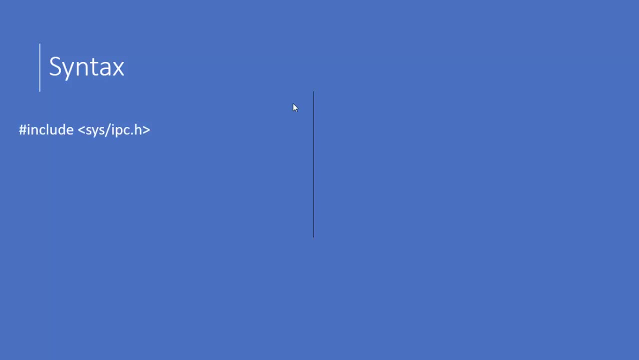 syntax of these two functions. so the header files required for shm get are sys ipc- dot h and sys shm- dot h. the shm get function will take three parameters. the first parameter specifies the unique number, called the key, which identifies the shared segment. so since you can create multiple shared segments, this key is going to identify each one of them. 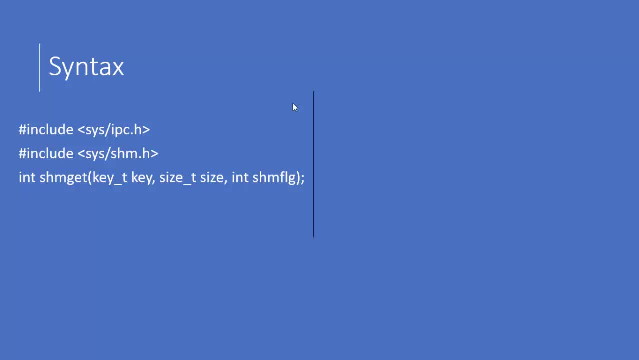 distinctly from the other. the second parameter is the size of the shared segment. the size will be specified in bytes, so you can give here 1024 bytes or 2048 bytes, whatever size you want to give the size of the shared segment. the third parameter specifies the permissions on the shared segment. so whether you want to 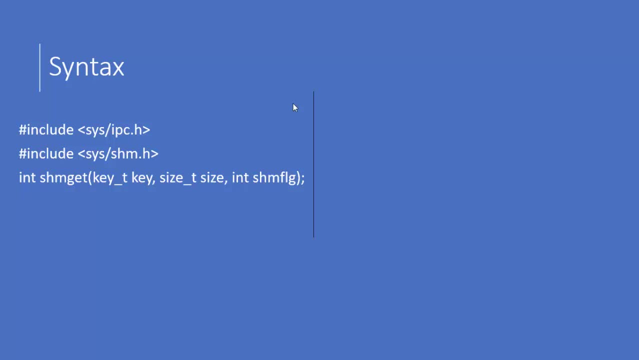 give read permission, write permission or both the permissions, whatever permissions you want to allow on that particular shared segment. on success: the schm get function returns a valid identifier which will be used in the next function, shm AT. so, whatever, the shm get function returns that particular integer. 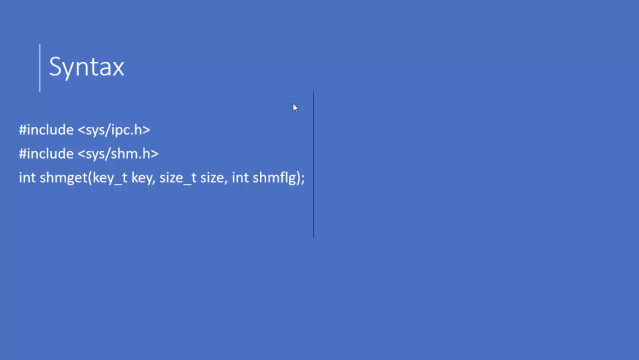 will be used to verify some hat Allegiances based on that obtentively selected value technique used by the shm80 function to attach the shared segment to the address space of the process. Now let us move to the second function, which is shm80.. So one of the header file is same- shmh, and another header file is sys slash- typesh. 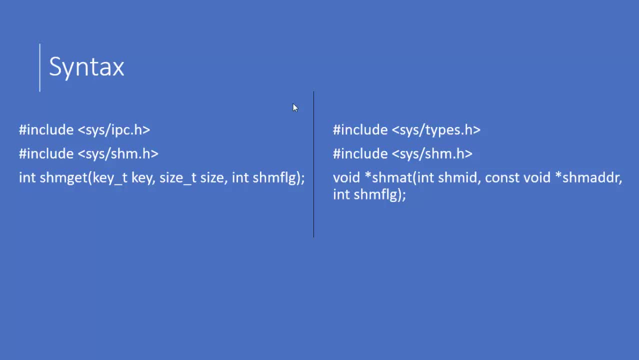 Now shm80 also takes three parameters. The first parameter is an integer type variable. Now this integer type is the value that is returned by the shmget function, So I will show you this in the program. The second parameter is the address where to attach the shared segment to the calling. 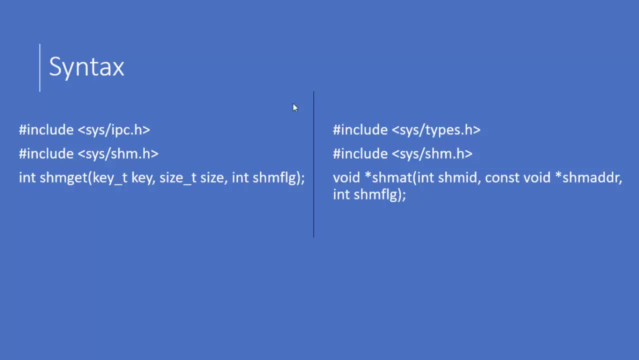 function To which point, in the address space of the calling function, either the sender or the receiver- The shared segment, should be attached. that particular address memory address will be given in the second parameter Now, since we don't know what is the addresses that are allocated to any process. 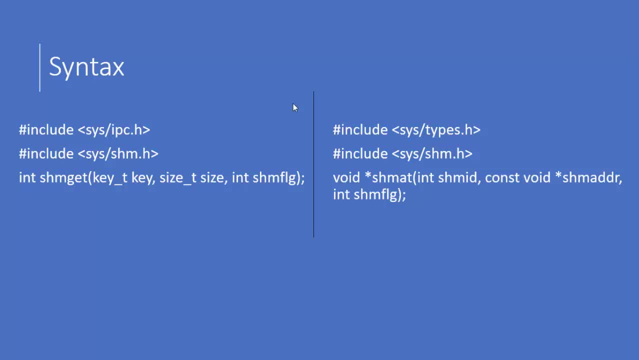 Hence we will write here null. Null means the system will automatically assign or choose a suitable address to attach the shared segment with the address space of the calling process. The third parameter is zero If the second parameter is null. Otherwise the value will be specified by another variable: shm. underscore rnd, in case you want. 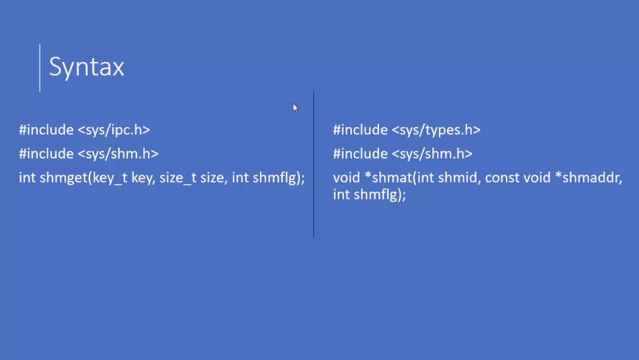 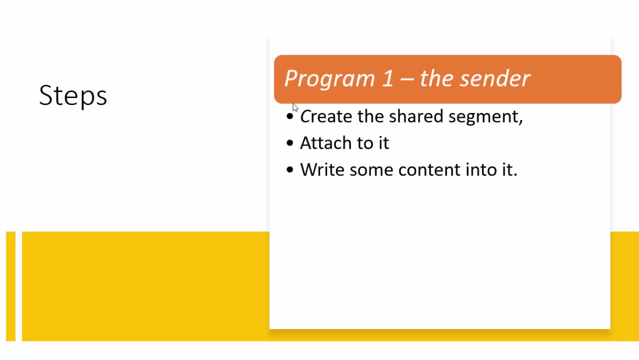 to give the address specifically by yourself. So we will not get into that. Just let us keep it very simple. So we will take the second parameter as null and the third parameter as zero. So we will write two programs. The first program will be the sender process. 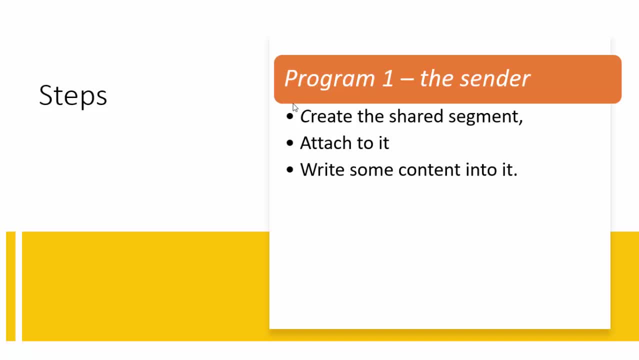 Which will create the shared segment, Attach itself to it and then write some content into it. So the sender program will contain three steps: Creating the shared segment, attaching to the shared segment and writing some content into it. The second program will act as the receiver. 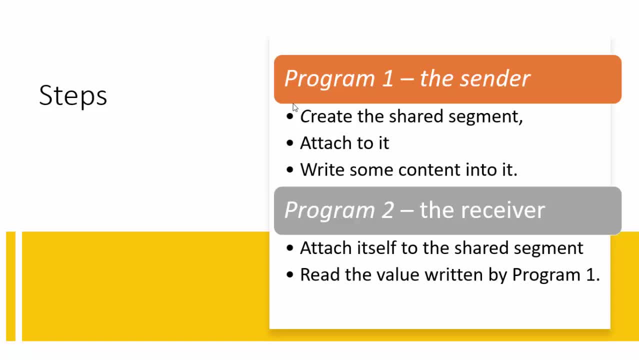 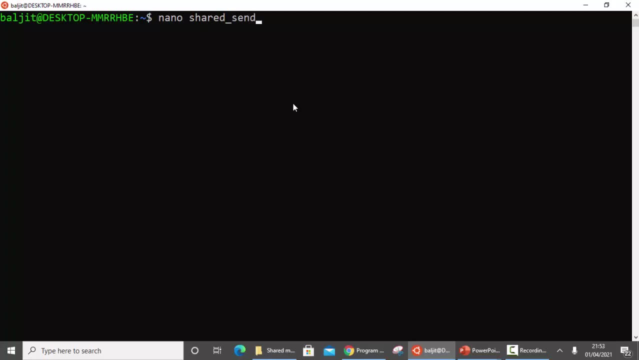 In this we will first attach the process to the shared segment and then read the value that was written by program one. Now let us look at the programs. So My first program is the sender program, So I have named it. shared underscore: sender dot c. 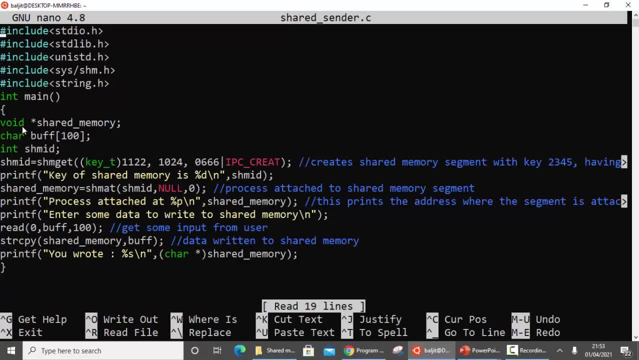 So the header files are there. The first variable I have taken is shared memory. This variable I have taken to store or to print the address where the shared segment gets attached to the process. address space Buffer is used to get the data from the user. 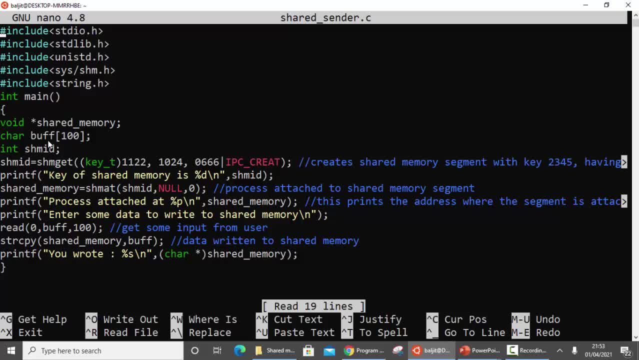 So that I can write it into the address space, into the shared segment, And then I have taken a integer variable. So the very first step is to create the shared segment. So to create the shared segment, the function is shm- get, So shm get first parameter was the key. 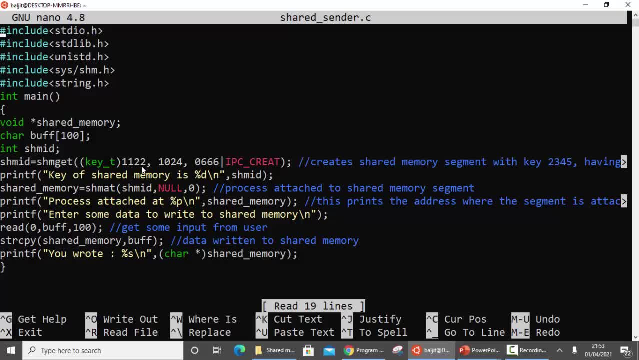 So I have given the key as one, one, two, two, So you can give here any number, whatever key that you want to assign, any number that you want to assign to the shared segment. Second is the size. So I have created this segment of one, zero, two, four bytes. permissions I have given read and. 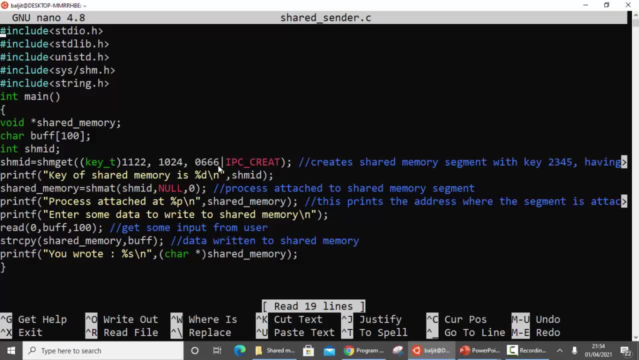 write to the user group and others, since we are going to create the segment, So we need to write IPC underscore create. So what this function is going to do, this is going to create a shared segment whose identifier is one one two, two, size is one zero two four bytes and read, write permissions. 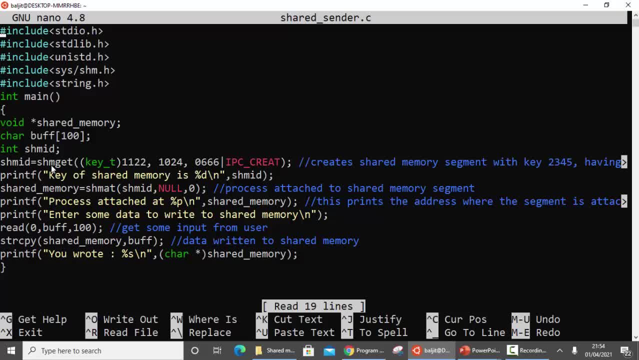 are available for everyone. The shm get function On success is going to return identifier which will be saved in shm id. This shm id will be used as the first parameter in shm at function. Alright, so the next step. I have simply printed that the key of the shared memory is so whatever. 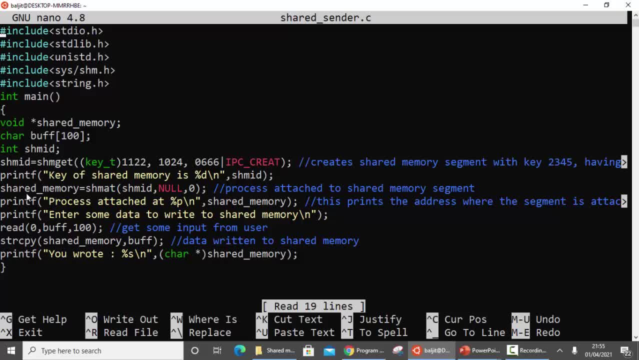 shm id value gets. so I'm just going to print that. Next we are going to use the shm at function, So the next step is to attach the shared segment to the address space of this process. So the first parameter is shm id, so which we have got from the shm get function. 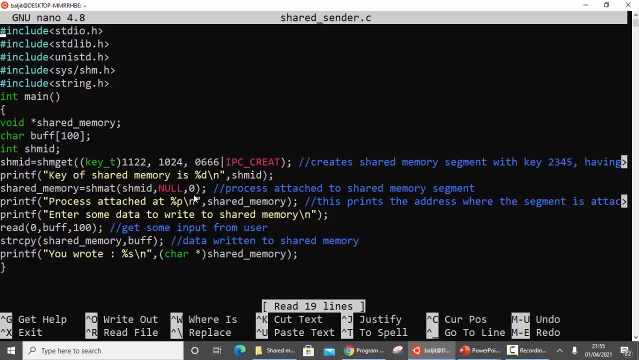 Second parameter, as I have told you, will be null and the third parameter will be zero. shm at function will return the address space or the address where the segment gets attached to the process. So I have printed that here for you in the next line. 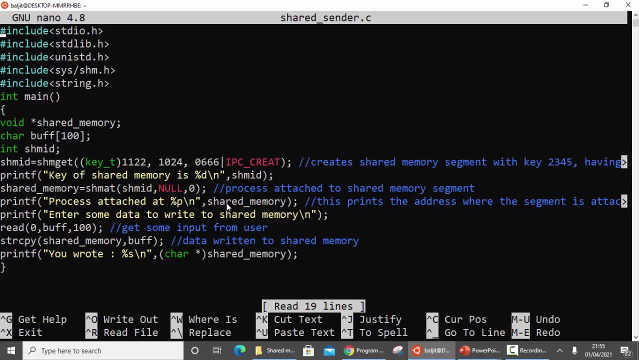 Process attached at. and then I have printed the value of the address: ok, memory address. Next, I am going to write some data into the address space. ok, into the shared segment. So simply enter some data. so a popup for the user to enter some data. 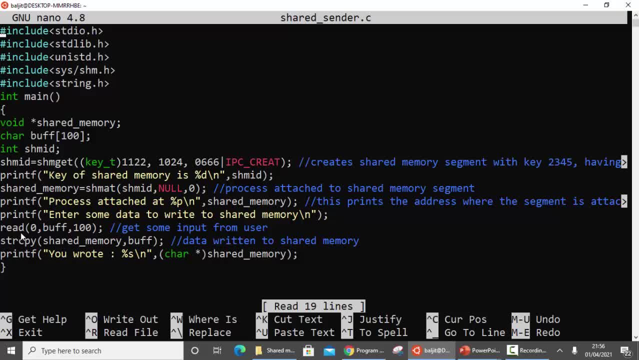 Whatever the user enters, I am going to use the read function to store that into the buffer. So read from the keyboard into the buffer: Alright, How much maximum funder. so the user can type maximum funder address. Last step is to copy this data into the shared segment. 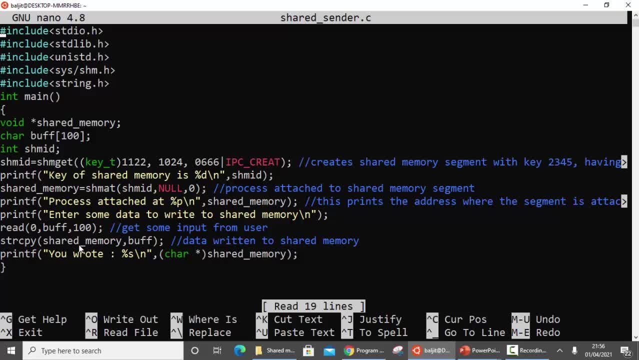 So I have used this string copy function: String copy copy where into the shared segment, from where? from the buffer. So whatever the user has written into the buffer is copied into the shared segment and I have simply printed whatever has been copied for the user to check. 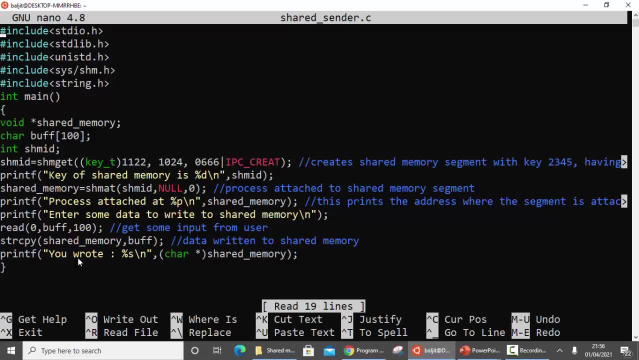 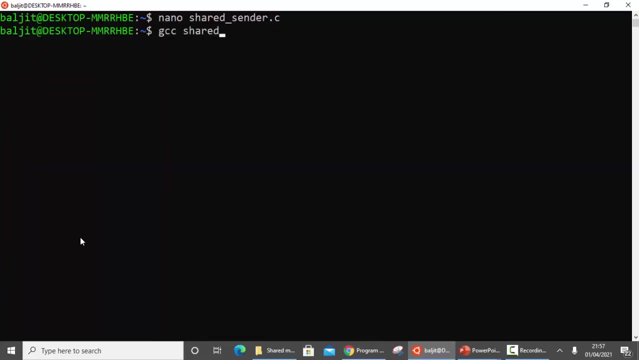 Ok, So we have done four things: First was to create the shared segment. Second, to attach the shared segment with the address space of the process. Third, to get some data from the user. and fourth, to copy that data into the shared segment. So let us now compile this gcc shared sender dot c and now run it. 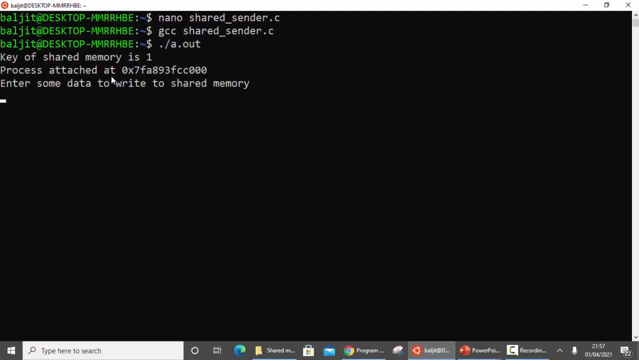 So you can see, here the key is 1. Process attached at. So this is the address where the process gets attached to the shared segment. Now it is asking the user to enter some data to write to the shared memory. So let us suppose this is a test program. 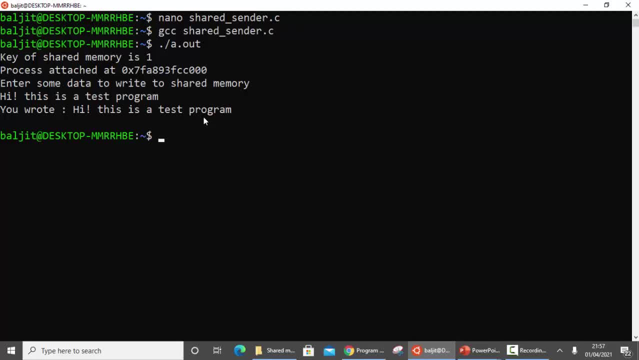 So this is the data which is written by the sender process into the shared segment. Alright, So the sender has sent the data. Return the data into the shared segment. Now my second program is the receiver program, which will receive or read whatever was written. 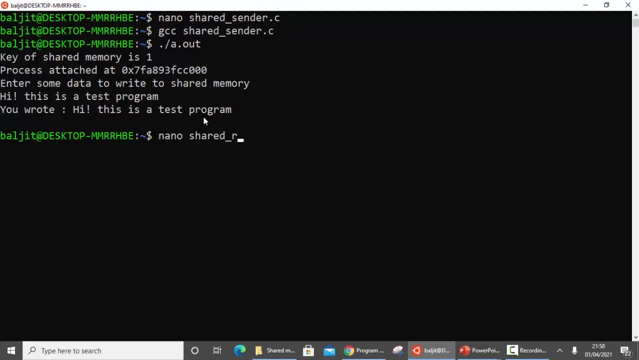 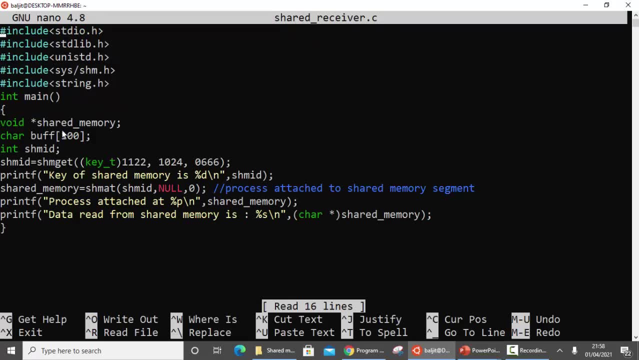 So this exact data should be read by this receiver process. Alright, So same variables I will require here also. In this program we are simply going to do three things. First, shm get. I need to use this function here also Because we need to get the shm id. 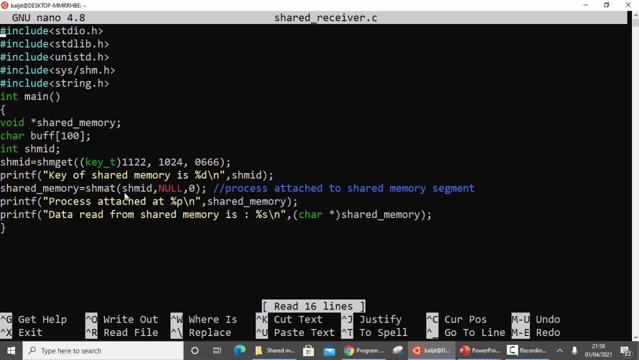 The id which we require as the parameter of the shm at function. Okay, So why I am going to use shm get? because we need to attach this process to the shared segment. For attaching the shared segment to the address, we need the first parameter, which is the return. 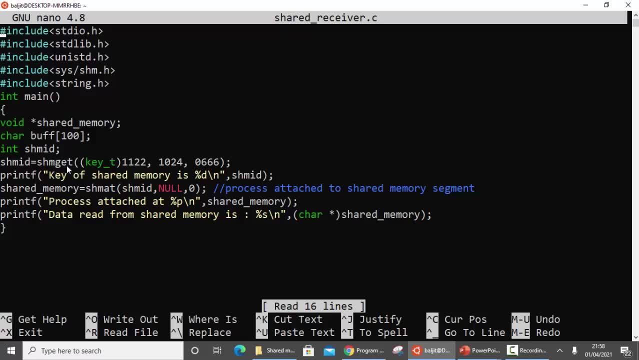 of the shm get function. So we need to call the shm get function, Write the same key, the same size, the same permissions. But the only difference is- I am not going to write here- ipc underscore create, because the segment is already created. 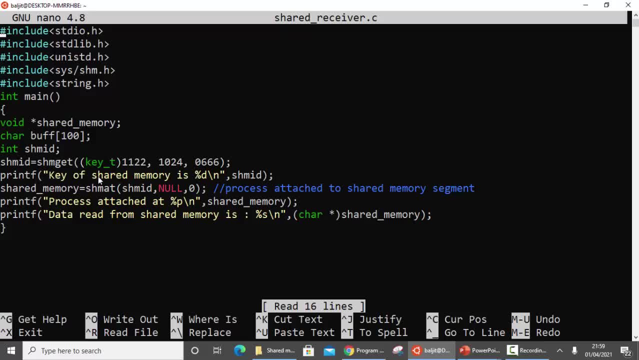 So we will get the same id. Then we are going to use that id in the shm at function. So you can see that this shm at function is exactly the same, But this time since it is going to attach to a different process. So this time, since it is going to attach to a different process, 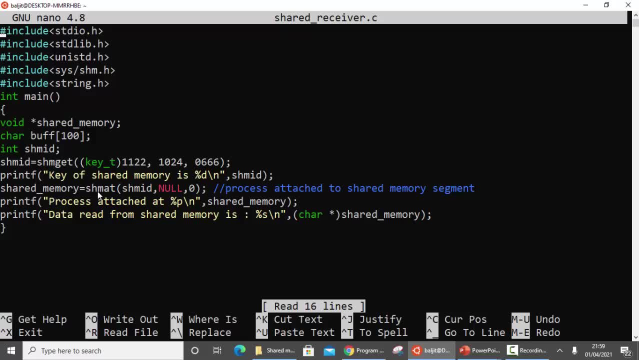 So this shared memory value will be different. Why I am using shm at? because I will attach the shared segment to this receiver process, which is another process, So it will attach itself to the address space of the receiver process. now, Once it is attached, I am simply going to print the data from the shared segment. 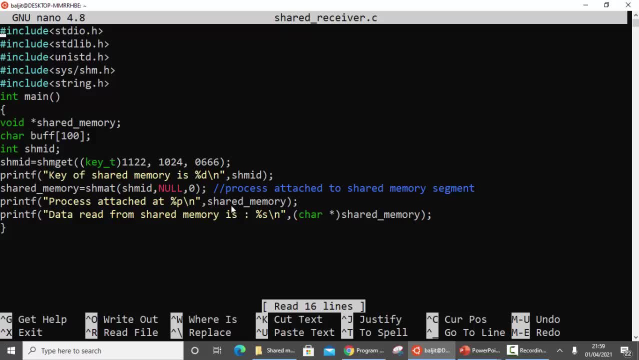 So you can see here printf process attached. So I will print the address here And next I will read the data directly Using the printf function. data read from shared segment is start reading from the starting byte of the shared segment. So here what I am doing is I am reading whatever is there in the shared segment, starting from: